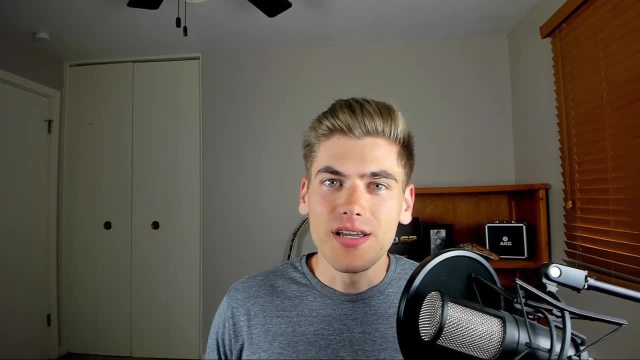 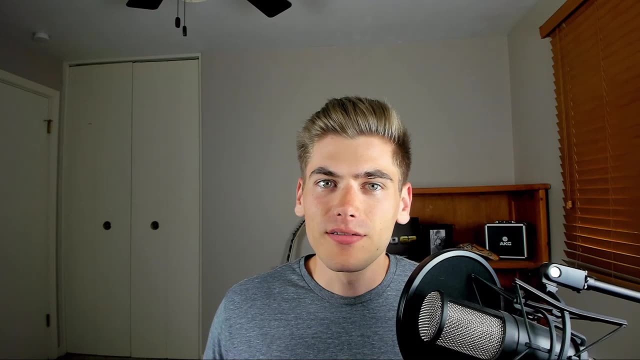 One of the greatest things about React is its ability to manage your data and properly re-render your application when your data changes. But there are two main ways in React to think about data. There's props and there's state, and it can be a bit confusing to understand when you 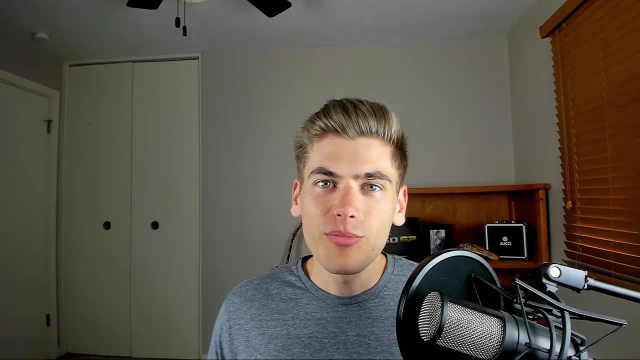 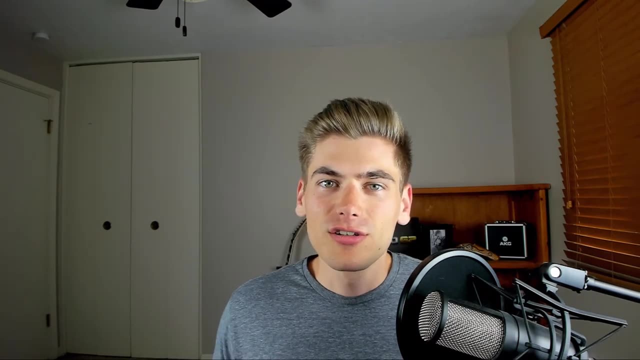 should use props and when you should be using state. So in this video, I'm going to break down exactly what props are, exactly what state is and why you should use props versus state inside your application. So, without any further ado, let's get started now. 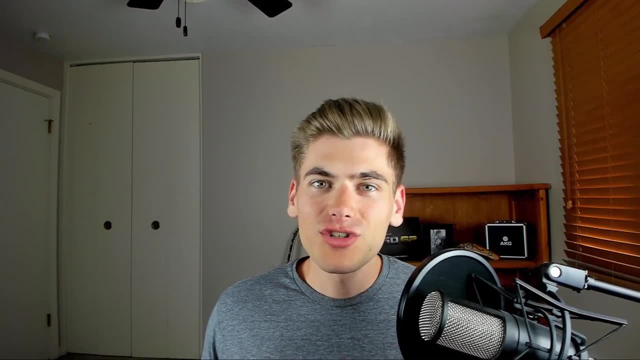 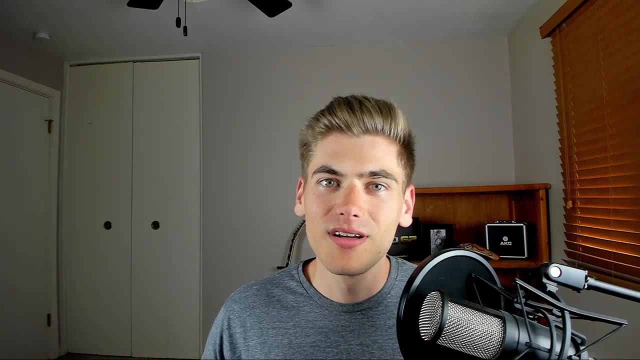 Welcome back to WebDev Simplified. My name is Kyle and on this channel I'm here to simplify the web for you, So if that sounds interesting, make sure you subscribe to the channel for more videos just like this one. Now to get started, I want to break down exactly how you use props and 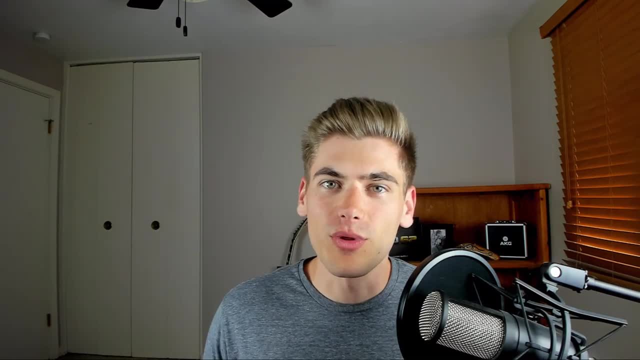 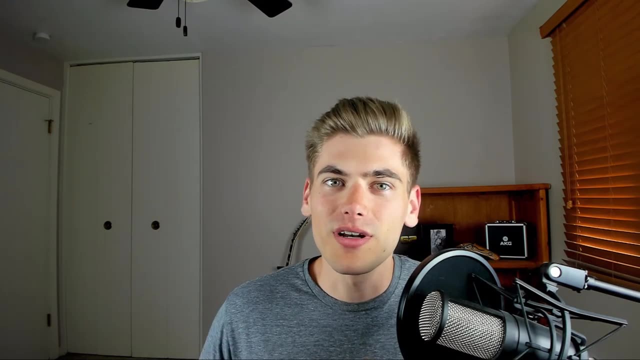 how you use state and what each of them is. So first we're going to start with props, And props you can think about as like arguments to a function. When you create a component inside of React and you want to render it, you're going to pass it the props that you want to give to it. 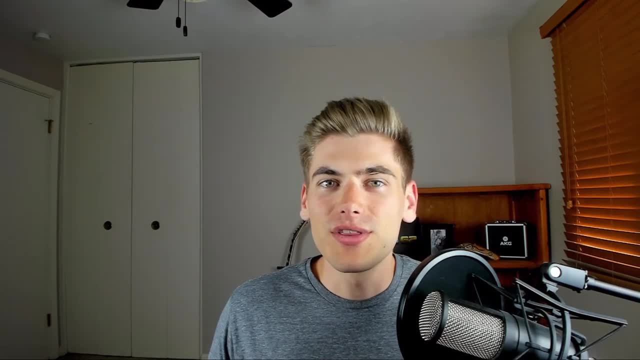 For example, let's say you want to render a component inside of React and you want to render it the props that you want to give to it. So let's say that we have a counter application. The thing that you're most likely going to pass to that counter is going to be the initial count. 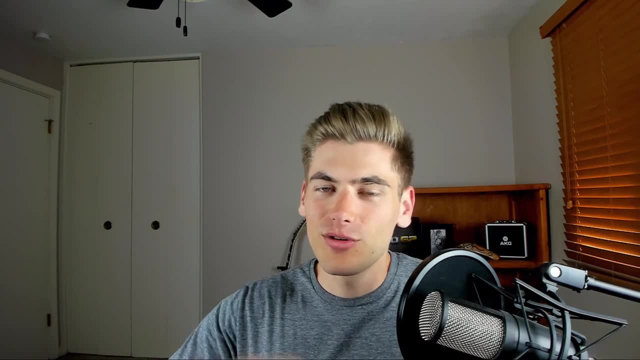 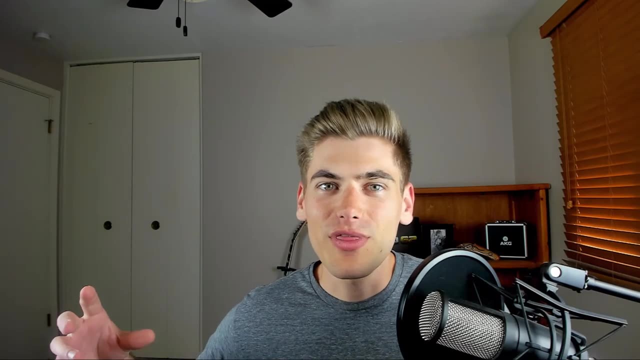 essentially what your count should start at. So you're going to pass your counter component its initial count inside of the props, And the reason we're using props for this is because props is kind of for things that you pass to like a function. They're what you want to initialize. 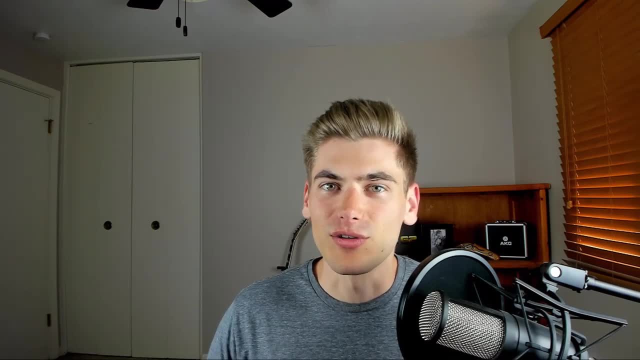 your component to or what you want your component to render like. So in this counter example, we want our initial count to be zero, So we're going to pass that through in the props. Something you can think of where you might need props is, let's say that you want to display something to. 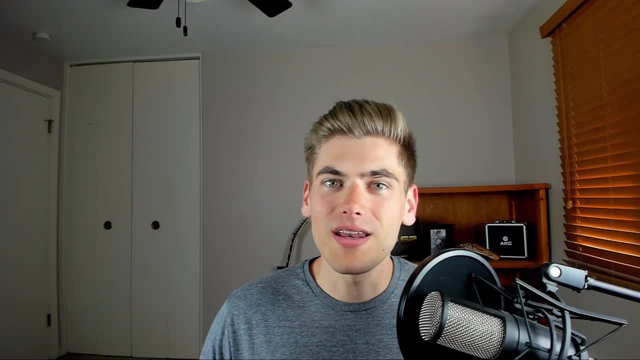 the user that has a title and a subtitle. You're going to also store that in the props, because what you want your function or your component to actually take is going to be the props. In our case, our component is storing a title and a subtitle, So we're passing those through the props. 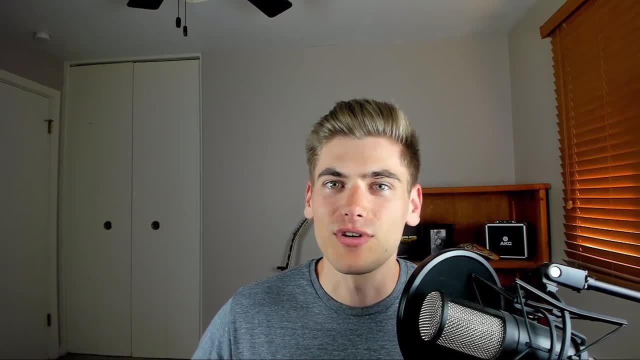 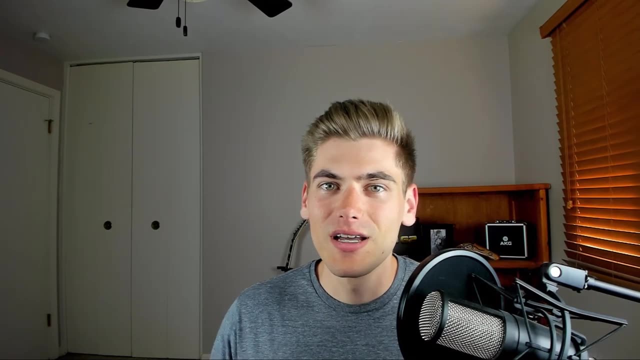 and then our application knows if those props change at some point. So, for example, something else in our application changes those props, It'll re-render that component for us, because our props are now different, But state, on the other hand, is quite a bit different. State is something inside of a component. So the big difference 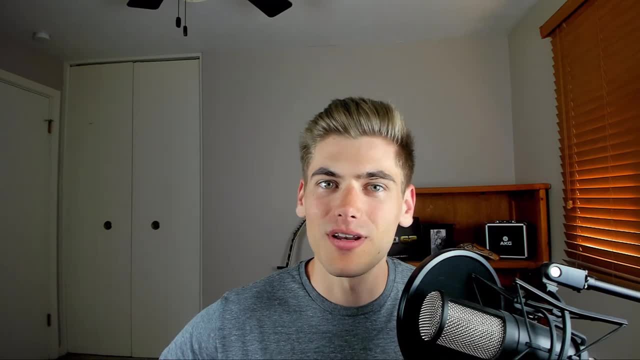 between props and state is: props you pass into a component and state is handled inside of that component and props are handled outside of the component. So in the example of our counter application, your current up to date count is handled inside of the state. So while we pass, 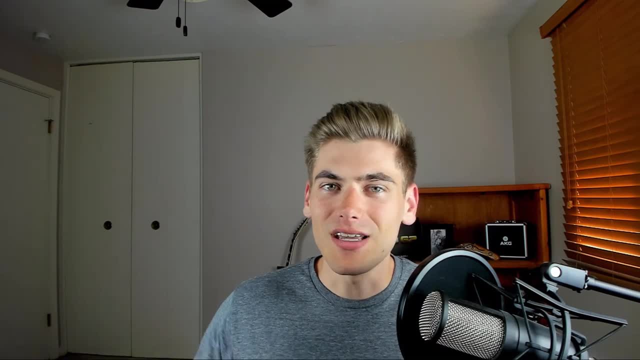 in the initial count. in our props we're just setting our state to that initial count And then inside of our component, that's handling our counter. we actually manage updating our counter to increase it or decrease it depending on what the user does, And we're using state for that. 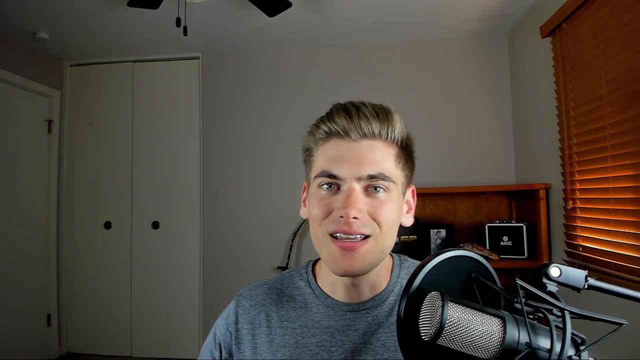 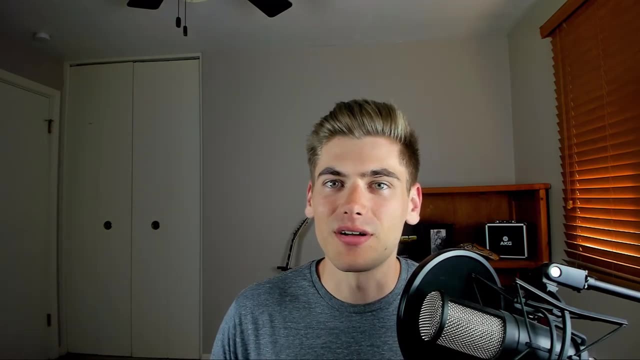 This is really the big difference between state and props. State is handled in the component and you can update it inside the component, while props are handled outside the component and must be updated outside of the component. Another thing about state versus props is when you change the 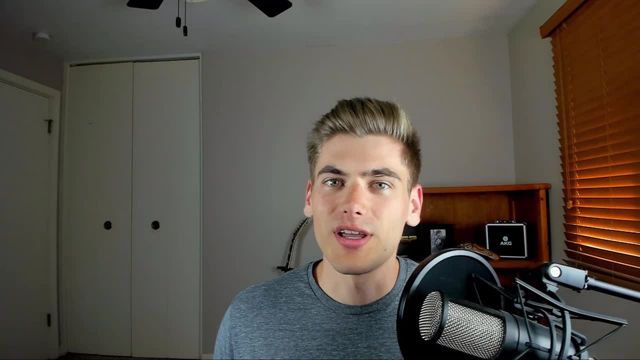 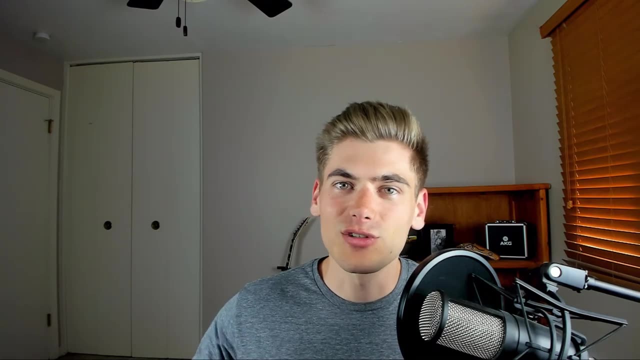 state inside of your application. it's going to re-render that section of your application, But props, you can't actually change them. You need to change them outside the component, like we talked about. Most likely it's going to be state stored. 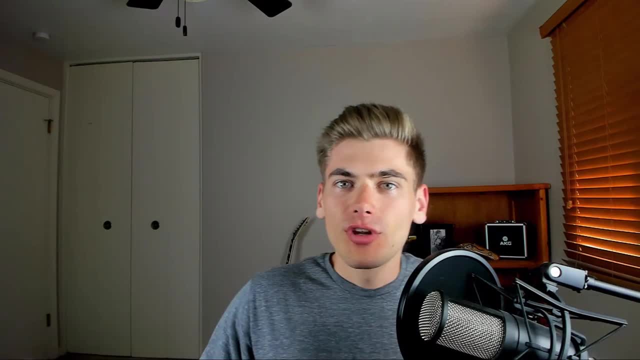 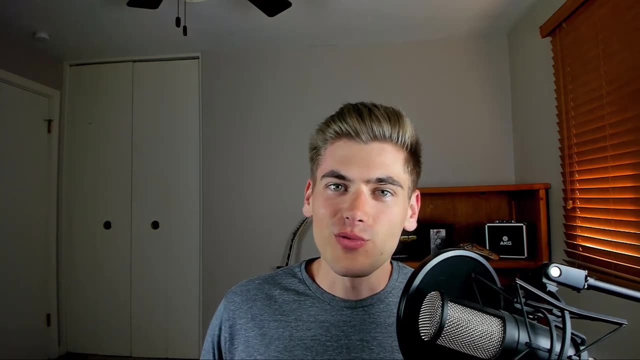 somewhere else in your application that's being passed down as props. Going back to our subtitle and title component, most likely this component is not going to have any state at all, because all it's doing is rendering some text and that text is never going to change. There's nothing in that component that can change, so it doesn't need any state. 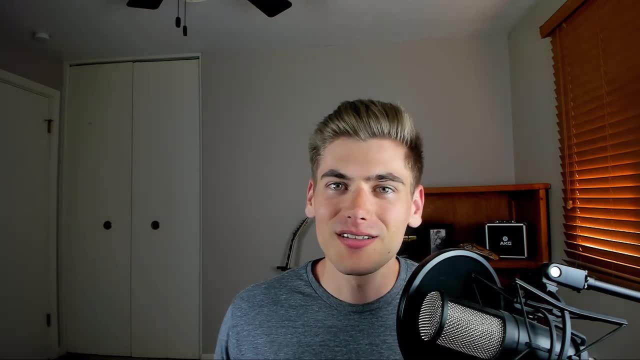 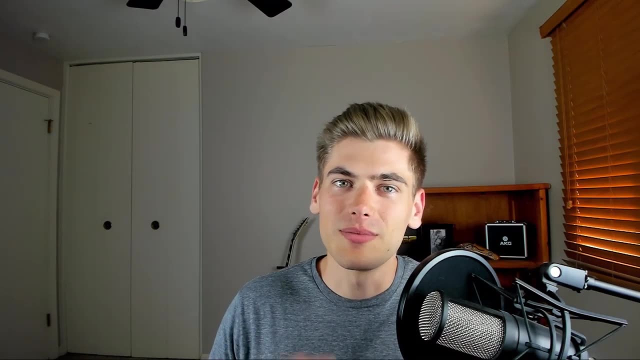 It's just going to take those two props and display them and that's all the component does, which is great. It's just super simple. But with the counter we're actually updating the count, So we need state to store that thing that we're going to be updating. And that's really where 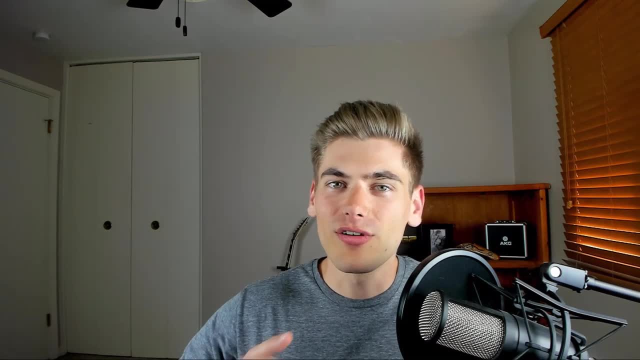 state comes in handy. So we're going to go ahead and change that. So we're going to go ahead and change that. So we're going to go ahead and change that. So we're going to go ahead. and state is there for when you need to actually rerender and update your application based on. 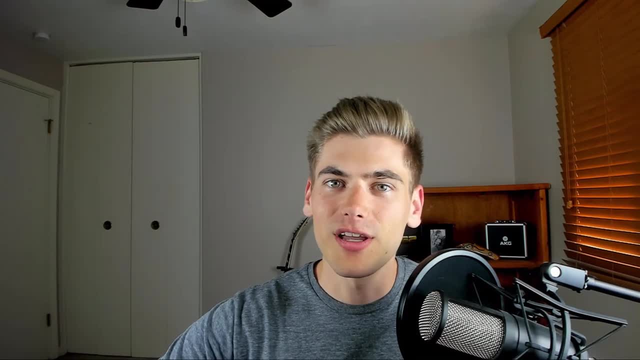 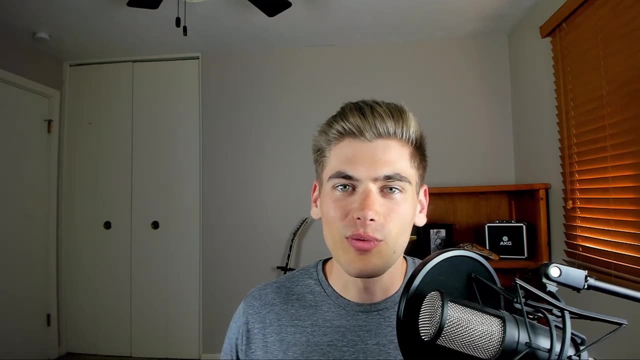 something the user has done. So if you want to change something in your application, you need to store that in state so that it properly rerenders when that actually changes. Props, on the other hand, are useful for when you want to display some information. 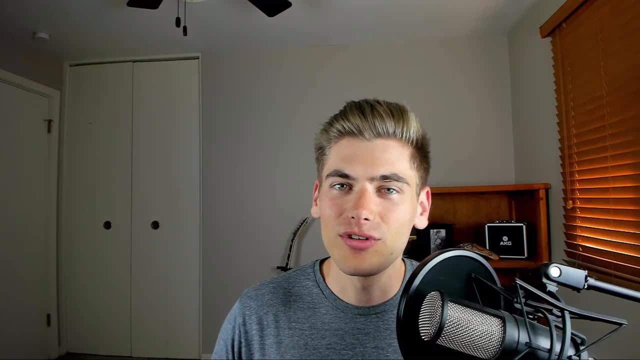 inside of a component without hard coding it. Essentially, it's a variable to a function. You can also think about it when you create a class with a constructor. the things you pass to the constructor of that class are going to be the things that are your props for a 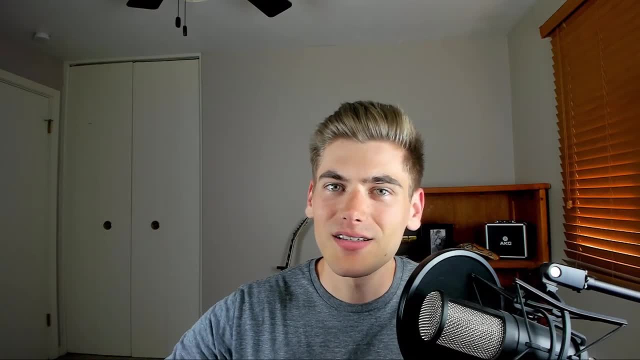 component. So that's why we're going to change that. So we're going to go ahead and change that component in React. So, for example, we're going to be passing that title and description down because we want to render those And we don't just want a component that renders the same title and 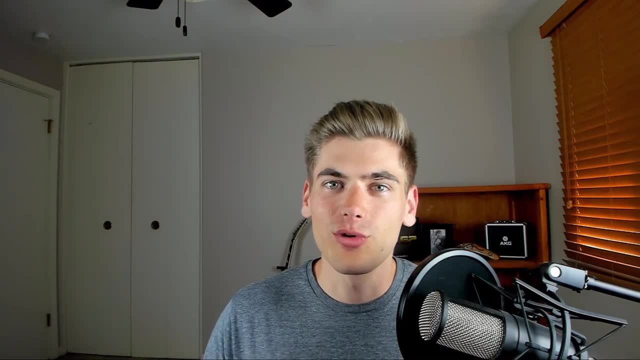 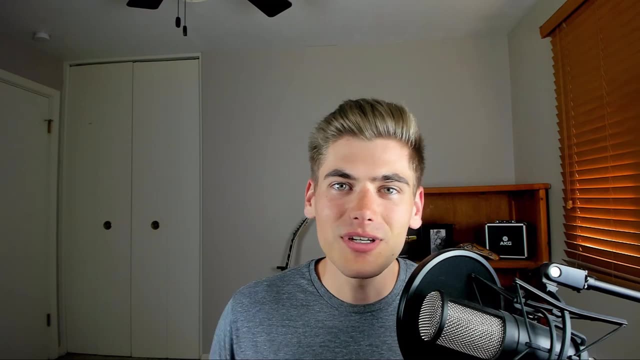 description. We want that title and description to be different, So we're going to use props in order to make that dynamic based on what we pass to that component. But with our counter application we have some count that we need to update inside of our state, So we're going to use state to make. 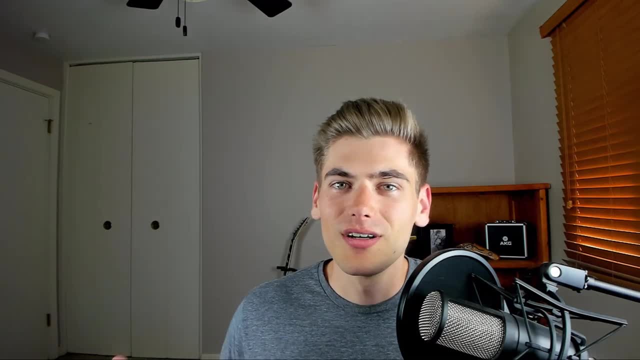 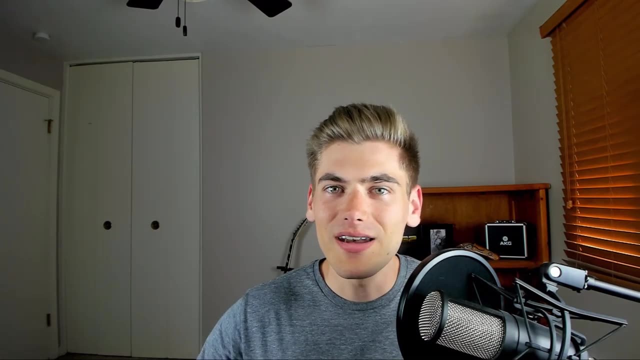 sure we continually are able to update that based on user input. Another example where state is really useful is inside of a form. If you have an input element, checkbox, select box, whatever it is- that needs to be able to be updated by the user. So we're going to actually use state to. 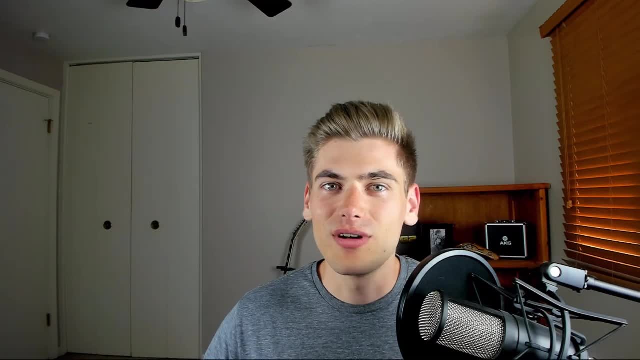 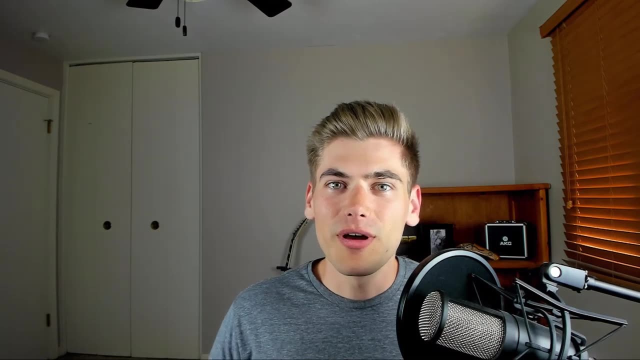 store what they're updating that value to and what they're changing that value to, and so on. The place where many people get confused when wondering when they should use state versus props is they don't properly think about which one is going to be handled by the component. 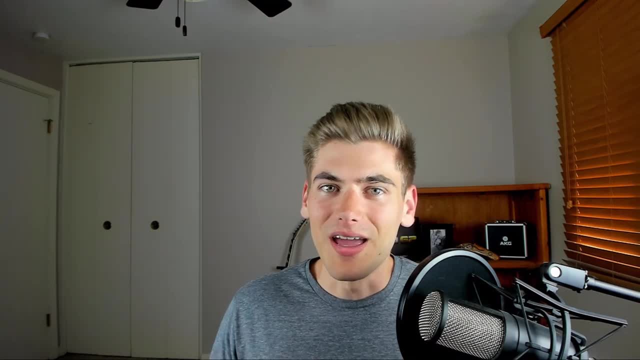 If you're handling that piece of information inside the component and inside that component, only nowhere outside of it, like in a parent, for example- then you're going to use state. If you're handling that information outside the component in, like a parent, for example- then you need to pass it in via props. Those are really the main differences. 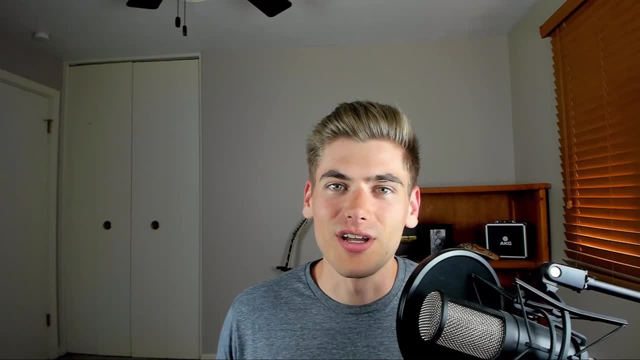 between the two. Also, if your information is static and not going to change, for example inside the component, you never need to update the title of that display section. then you want to use props, because props are for things that are going to be passed down from the 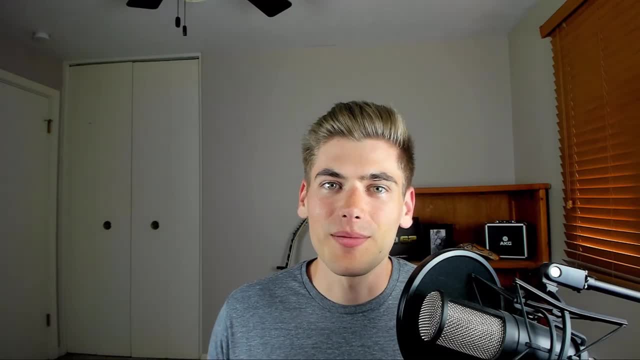 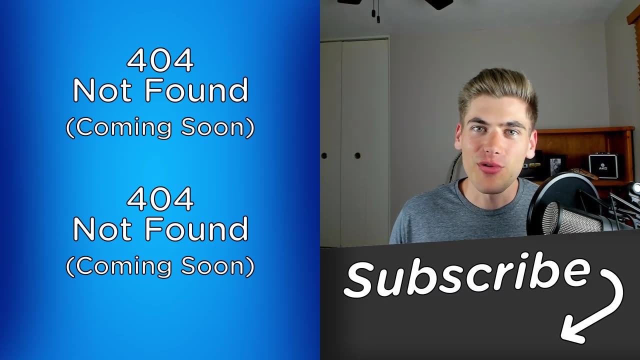 parent and don't change inside the component. But with the counter, like I mentioned, we're updating that in the component, so we need to use state And that's really the only differences between state and props. If you want to dive further into more details and nitty gritty of React, make sure you check out my 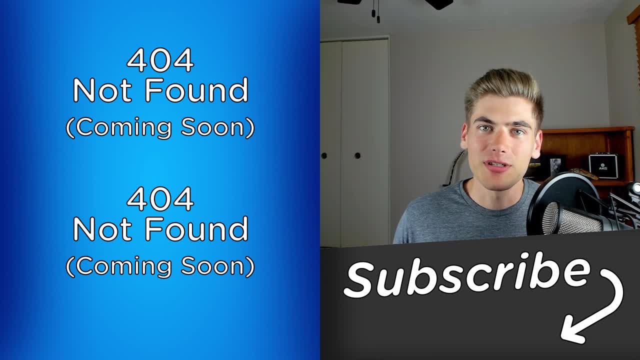 React course launching on September 10th, linked in the description and the comments below, And if you're coming here before it's launched, make sure you sign up for the email list where you can get an exclusive discount on the course when it launches. So with that out of the way, thank you. very much for watching and have a good day. 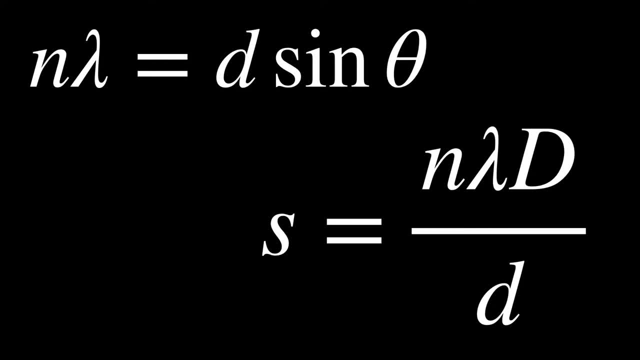 So in this video I'm going to derive the two versions of Young's double slit formula for the distance between maximums. The top formula gives an angular separation and the bottom one gives a distance s To first establish the conditions when this happens. we'll say that coherent light.